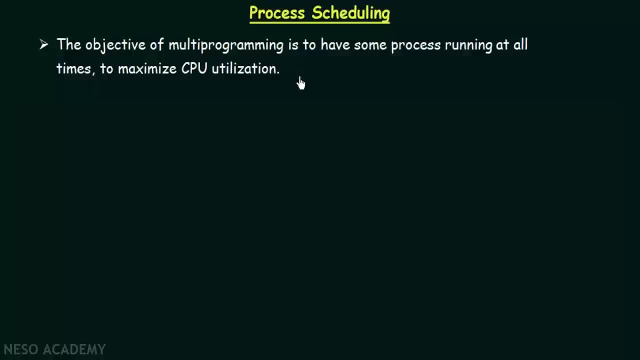 So we have already talked about multi-programming in the beginning of this lecture series, And the objective of multi-programming is to have some process running at all time to maximize CPU utilization. So what does this mean? So let's say that we have this CPU. 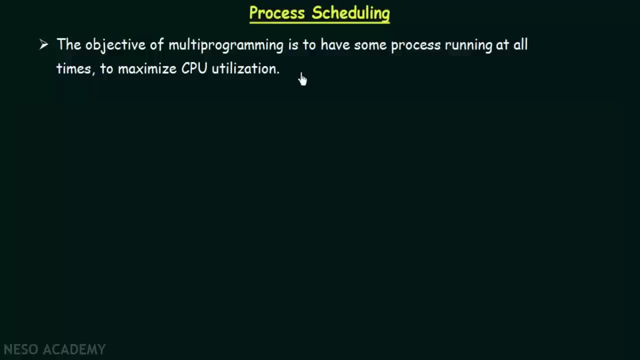 and let's say that we are using only some percentage of the CPU. Let's say that we are using only 20% or 30% of the CPU. So if we are doing that, we are not making complete utilization of the CPU. 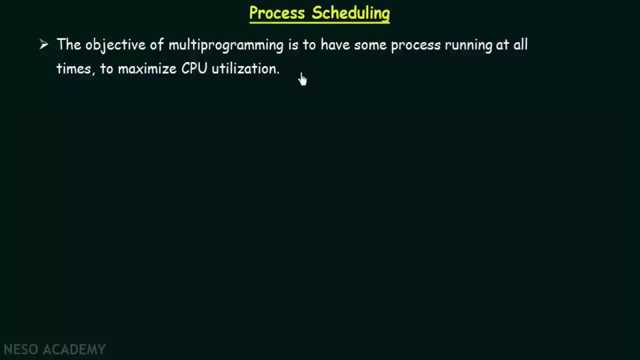 And hence we can say that we are wasting our resources. So the objective of multi-programming is to have some process running at all times. We want to have at least some process running at all times so as to maximize the utilization of our CPU. 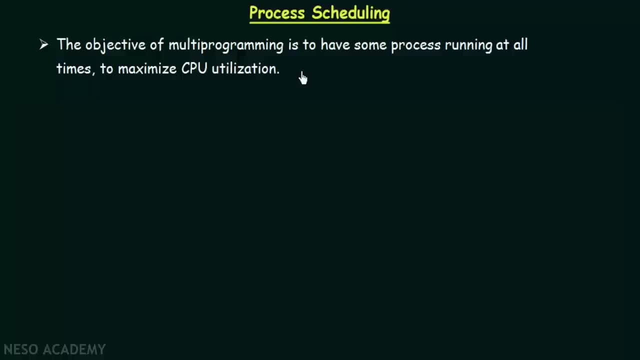 And hence we can say that we are efficiently using the resources that we are having. So that is the objective of multi-programming. Now you may ask: how is this related to process scheduling? Don't worry, we will come to that. 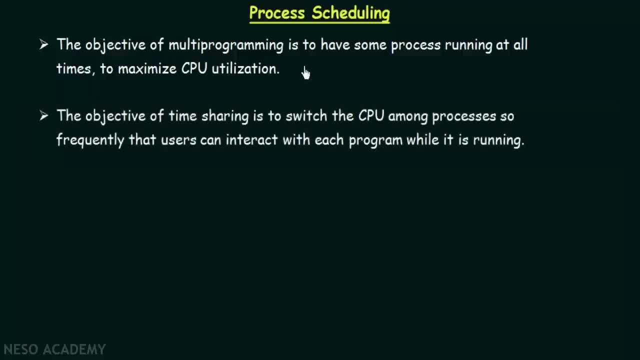 and you will understand how it is related as we move ahead Now. the next thing that we will be talking about is time sharing. The objective of time sharing is to switch the CPU among processes so frequently that users can interact with each program while it is running. 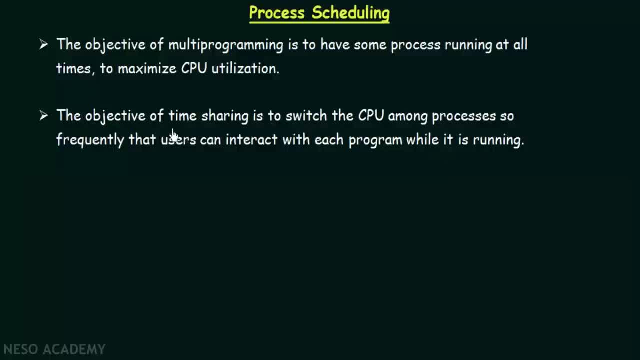 So time sharing is also something we have already talked about in the beginning of this lecture series, And the objective of time sharing is to switch the CPU among processes so frequently that users can interact with each program while it is running. So let me explain this using an example. 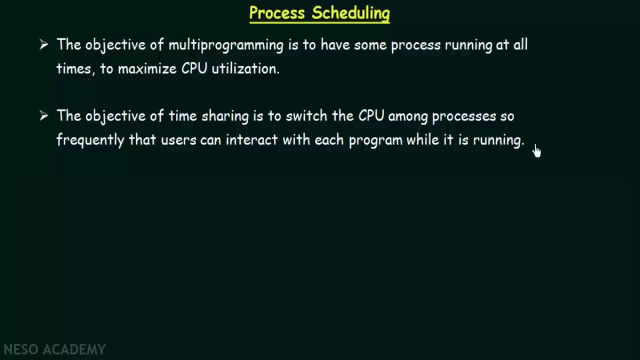 So let's say that in your computer you are typing a document using your Microsoft Word And at the same time you are listening to music using any of your music players, let's say Windows Media Player, And at the same time you are downloading some files. 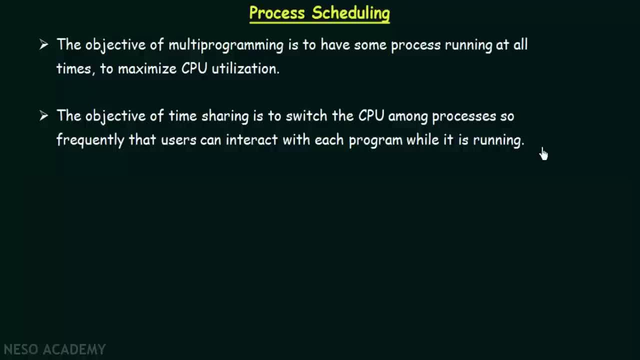 using your Chrome browser. So we see that you are able to do all these three tasks at the same time. You are able to type the document, at the same time you are listening to music and at the same time, the file is being downloaded in your browser. 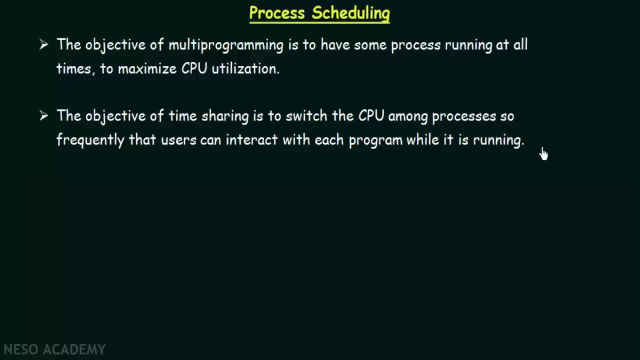 So we feel like we are doing these three things at the same time. But if you go deep into it and really look at it, we will find that these three things are not actually happening at the very same time. But what is happening is the CPU is switched. 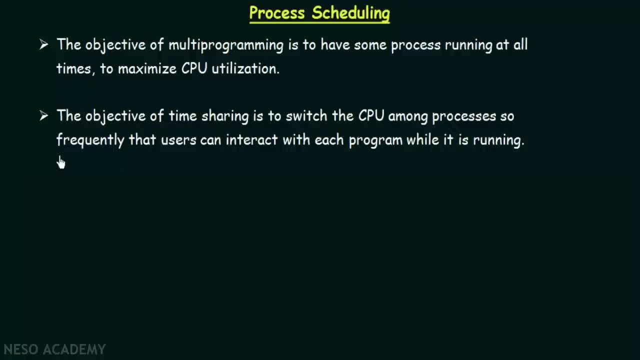 among these three processes so frequently or so quickly that you are able to actually interact with each program while it is running. So according to the human speed, if we look at it, we feel like these three things are happening at the same time, but actually it is not. 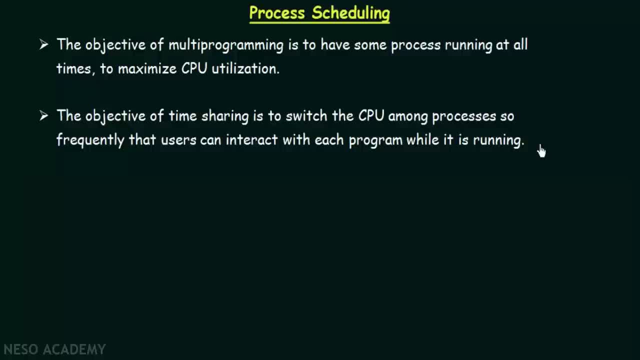 But the CPU among these processes are switched so frequently and so quickly that we don't actually realize that And, as a result, you are able to interact with each of these programs while it is running. Alright. so those are the objectives of multi-programming. 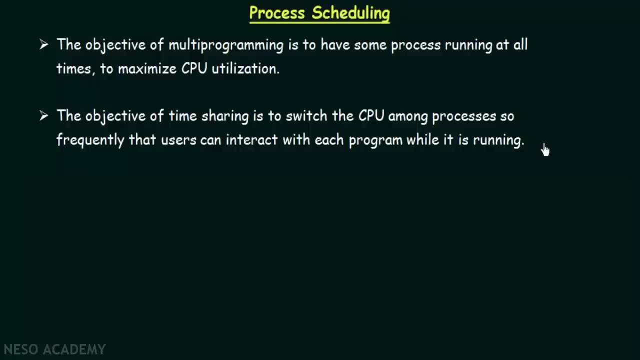 and the objectives of time sharing. Now, in order to accomplish these objectives, what shall we do? How are these two objectives accomplished? So, to meet these objectives, the process scheduler selects an available process, possibly from a set of several available processes, for program execution on the CPU. 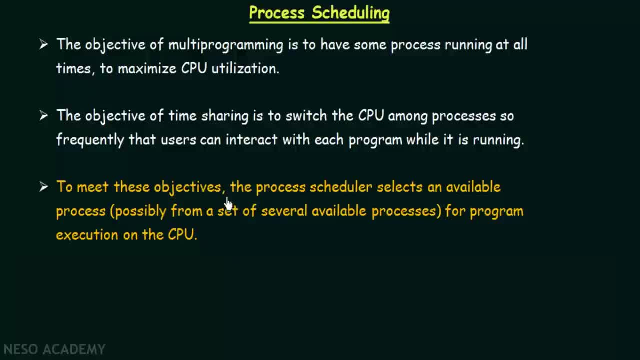 So, in order to accomplish these objectives, we have something known as the process scheduler, And what does it do? It selects an available process from the set of available processes that we have for program execution on the CPU, So we have several set of available processes. 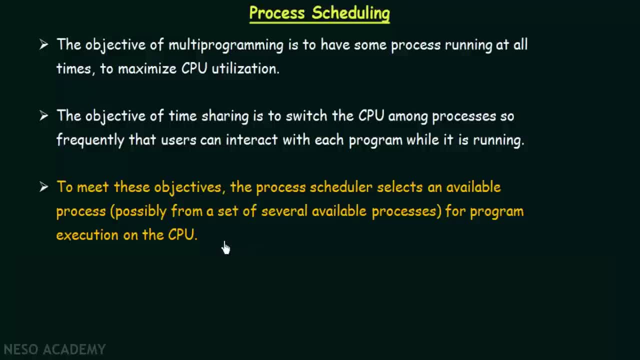 that are ready to be executed And the process scheduler will select an available process and it will assign the CPU to that process so that it can begin its execution. And what will happen when a process is being executed? Will it be allowed Or will it be given the complete time to complete its execution? 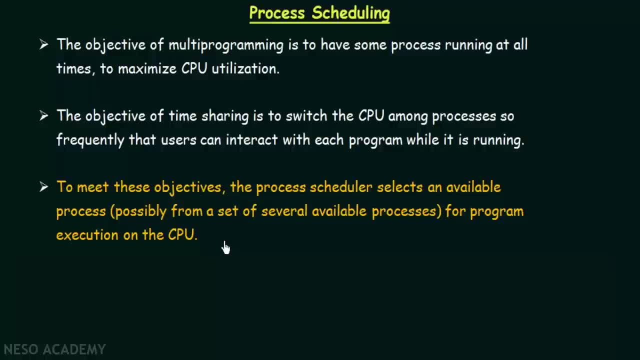 Or if another process comes with higher priority, will that process be given the chance to execute and the other one has to wait? All these things will be decided by the process scheduler. So that is where process scheduling is important and where it comes into play. 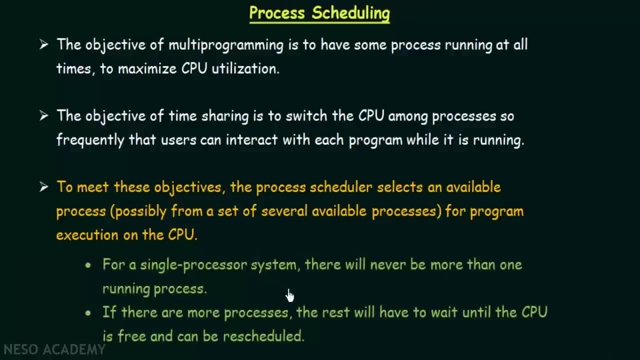 So, for a single processor system, there will never be more than one running process. If there are more processes, the rest will have to wait until the CPU is filled and can be rescheduled. So, as I told you, in a single processor system, 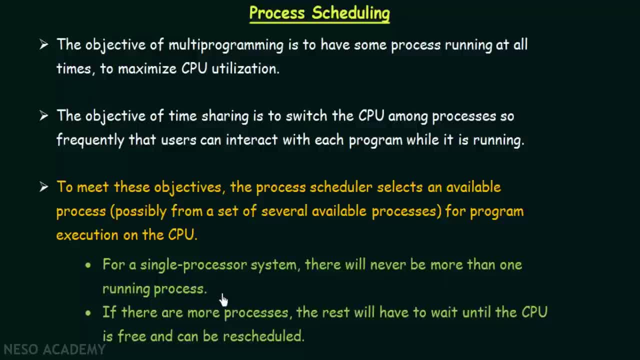 there will never be more than one running process. There will be only one single process running at a particular time. Though it may look like there are many processes running at the same time, but in a single processor system, only one process will be running at a particular time. 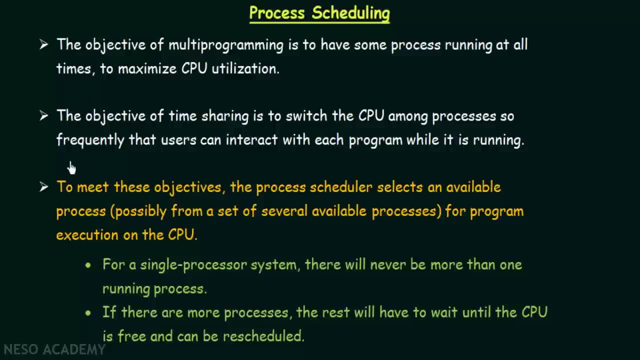 But what happens is the CPU is switched so frequently among these processes that we don't even realize that. And, as I told you, if there are more than one processes, then the rest will have to wait until the CPU is free and can be rescheduled. 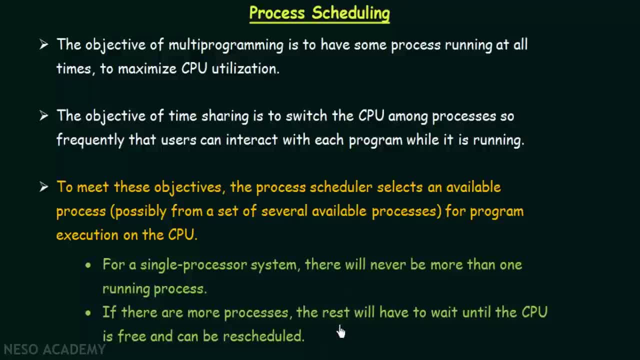 And who will take care of this. The process scheduler will take care of this, As of who will be executing or which process will be executing, and which of them will have to wait, and if higher priority process comes, then which will be executing. So, in order to help with this process scheduling, 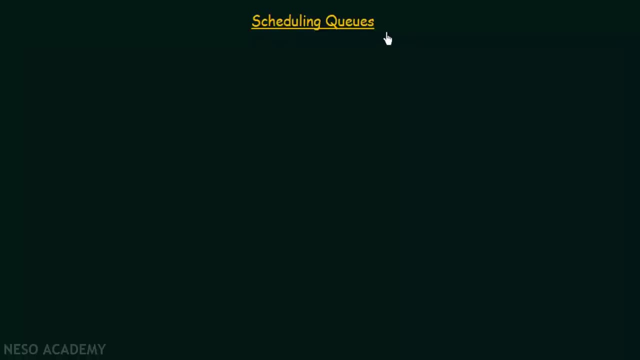 we have something known as the scheduling queues. So basically there are two kinds of queues, which are the job queue and the ready queue. So first we have the job queue. So what is this job queue? As a process enters the system. 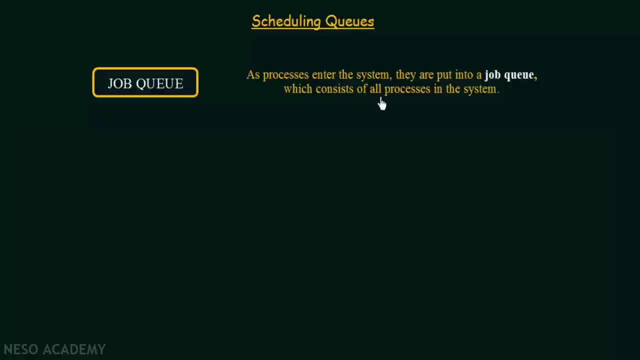 they are put into a job queue which consists of all processes in the system. So when the processes enter the system, they are put into a queue known as the job queue. So job queue consists of all the processes in the system. So they may not be executing at this time. 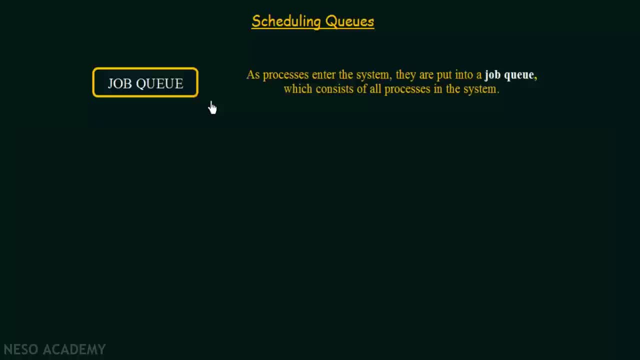 but these are the list or the set of all processes that we have in the system. So all these processes, they are put into this set or this queue, known as the job queue, where they will be waiting in order to go to the ready state. 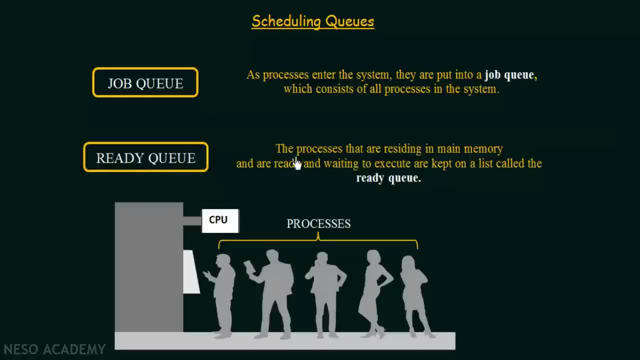 The next queue that we have is known as the ready queue. The processes that are residing in main memory and are ready and waiting to execute are kept on a list called the ready queue. So in ready queue we have those processes which are ready and waiting to be executed. 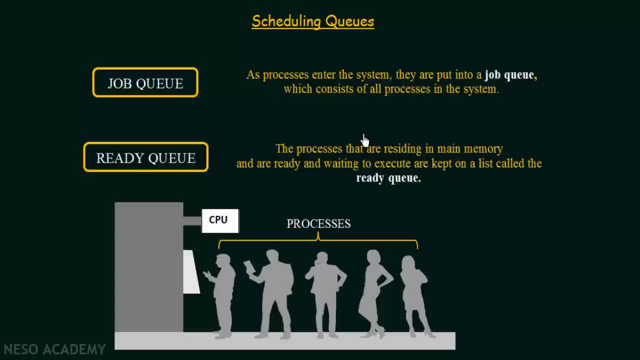 So these are the processes that are residing in the main memory and they are ready to be executed. They are just waiting to get the CPU so that they can start executing. So job queue is the list of all the processes that we have and ready queue is the list of processes. 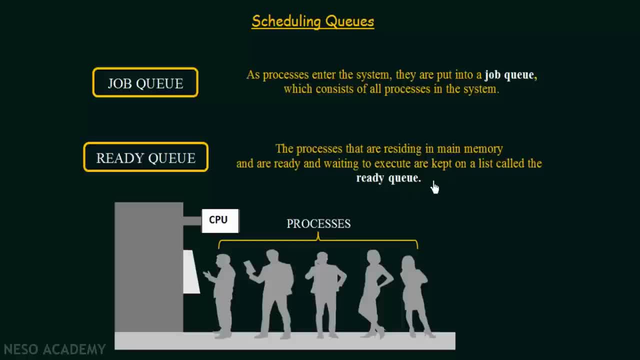 that are ready and waiting to be executed. So they are just waiting for the CPU and once they get the CPU they can start their execution. Now, once the processes are in the ready queue and once they receive or get the CPU for its execution, 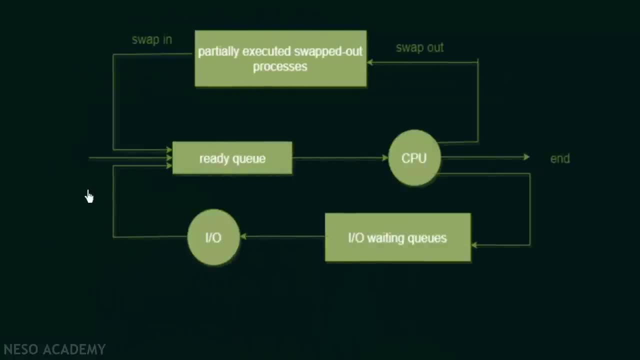 let us see what are the things that can happen. So this diagram here shows what happens to a process when it goes from the ready queue into the running state, That means when it gets the CPU, and what are the things that can happen. So here let us say that from the job queue, 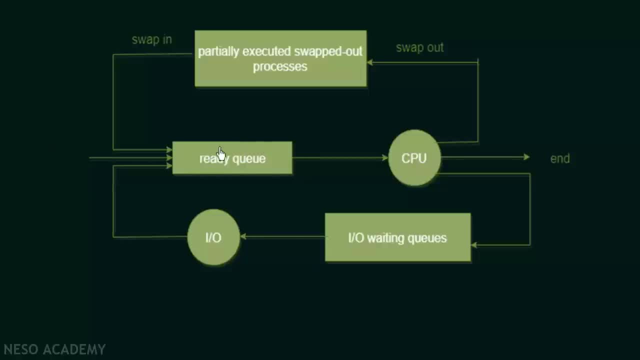 the processes, they come to the ready queue. So let us say that a particular process is in the ready queue and it is just waiting to get the CPU for its execution. So once it gets the CPU and it begins its execution, there are several things or several cases that can occur. 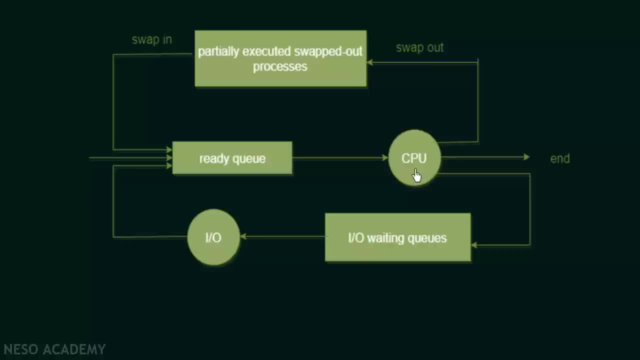 So the first thing that can happen is it received the CPU and it completed its execution and the process just ends. That means it goes to the terminated state. So there is one thing that can happen: From the ready queue it got the CPU. 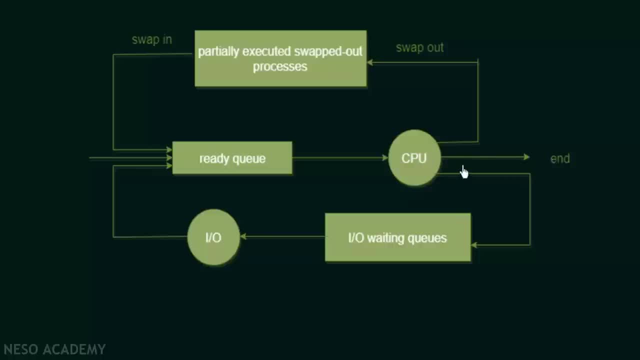 it completed its execution and it has ended. Now, another thing that can happen is it comes from the ready queue and it is assigned the CPU and it is holding the CPU for its execution. But at the same time, let us say that there is another process. 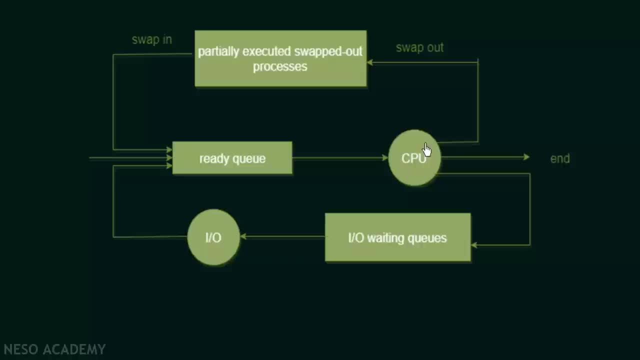 that comes with higher priority. That means this process that comes now is having higher priority and it has to be executed before this. So what happens? The process that was previously executing it will get swapped out and it goes to a list called the partially executed swapped out processes. 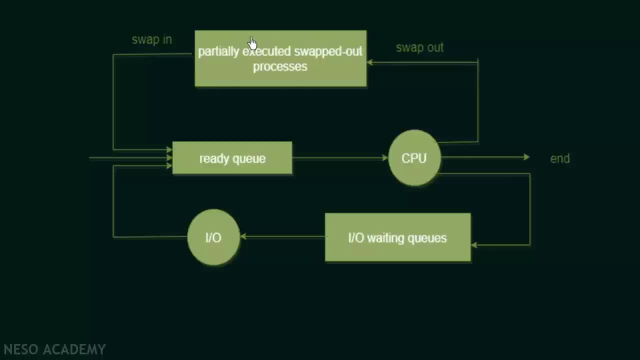 So it comes here, where it is swapped out, because another process of higher priority came and it has to be executed before that. So it is swapped out and it comes over here And after that it gets swapped into the ready queue again. 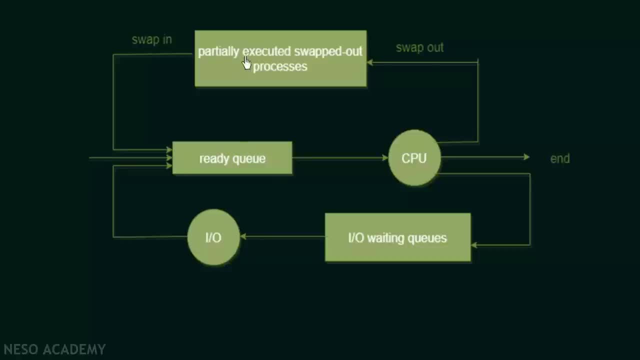 So the execution has not completed fully, It is just partially executed. So it still needs the CPU to complete its execution. So it comes back to the ready queue again waiting to receive the CPU. So it waits for its turn and according to the process scheduler, 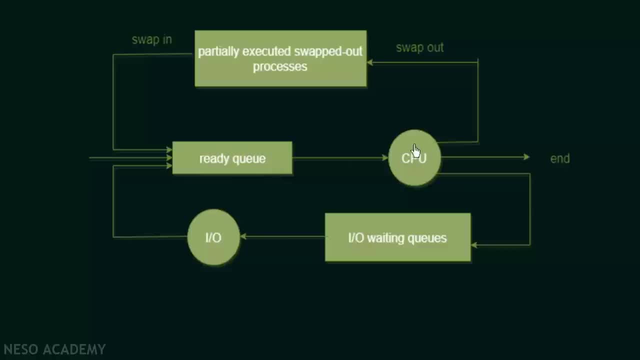 when it is assigned the CPU again, it will come and it will get executed, and when it is completed it will go to the terminated state. Now another thing that can happen again is from the ready queue it is assigned to the CPU and it begins its execution.